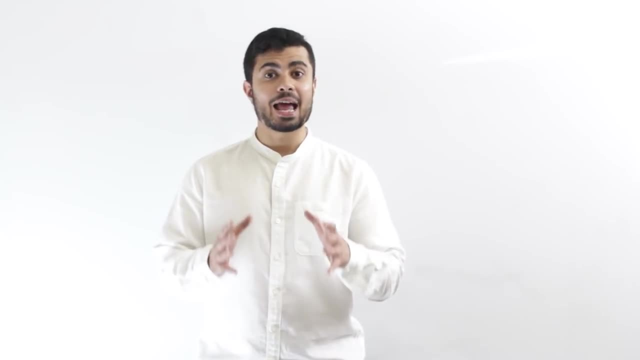 Hey guys, really excited for today's video because it's about dynamic programming. The question is that if you're given a matrix with ones and zeros, how do you find the largest possible square made of just ones? Now the problem may seem a little complicated. 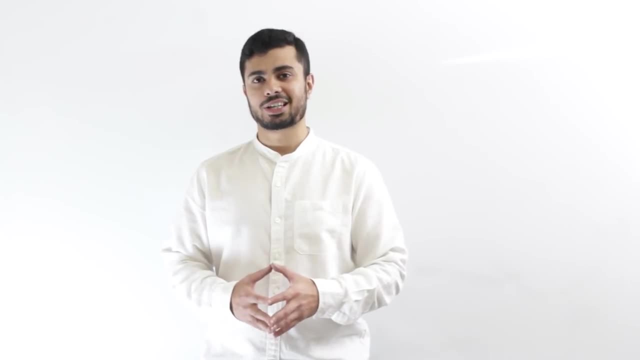 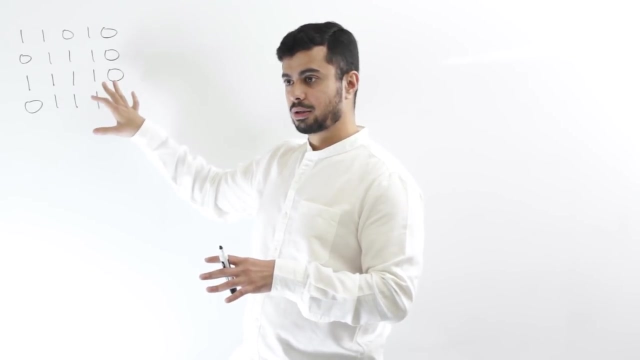 but just watch till the end at how simple the implementation is, So let's dive right into it. So we have this matrix and I have to find the largest possible square made by just ones. Yep, Okay, And the matrix can be of any dimension. Yeah, Okay. So in this example, 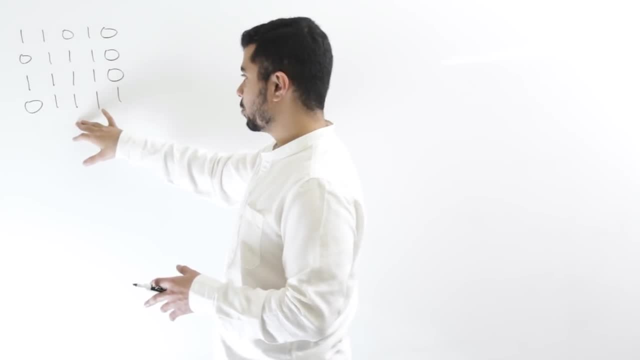 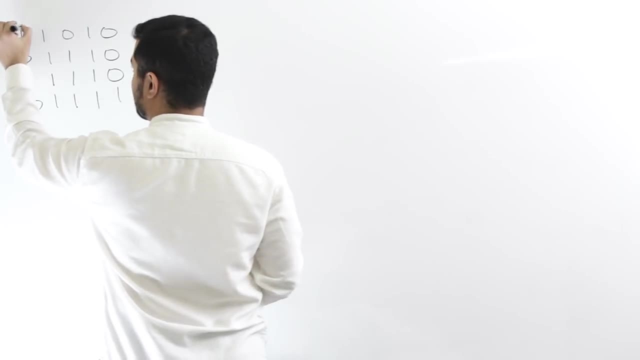 then the answer would be three, I'm assuming. Yeah, And also any index. which, for example, largest possible square for this particular index- let's say this index is the top left, corner right- Would be one which is just itself right. Yes, Okay, Perfect, So the first. 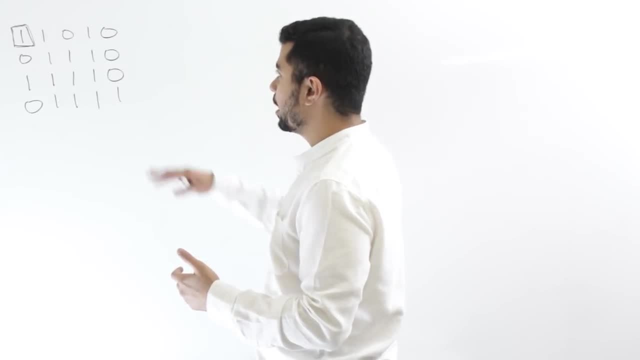 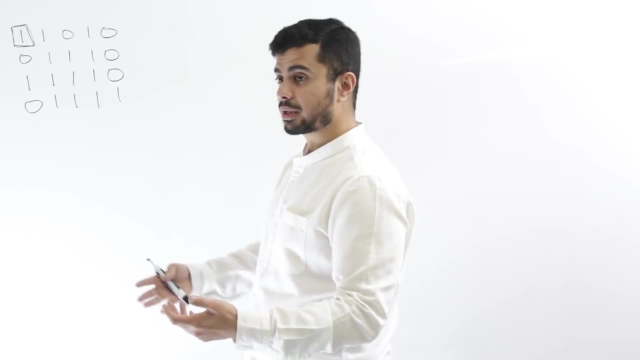 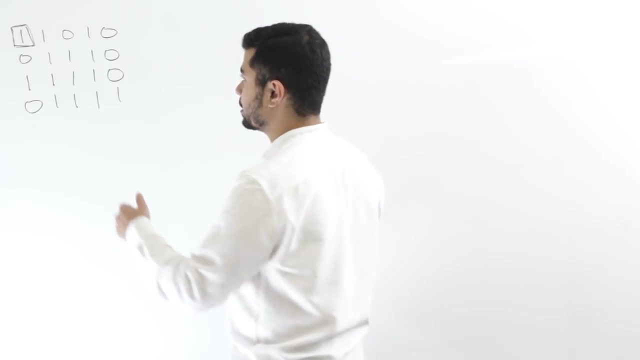 solution that comes to mind is: perhaps I can iterate through this entire matrix and find, find for each individual index what is the largest size. Okay, But that would be very inefficient. So the second thing is we just- I just mentioned that this is a top left corner- 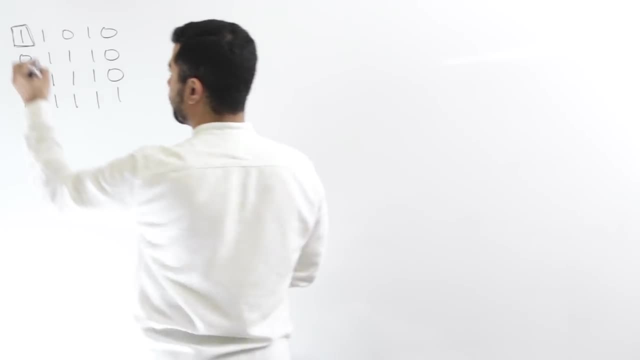 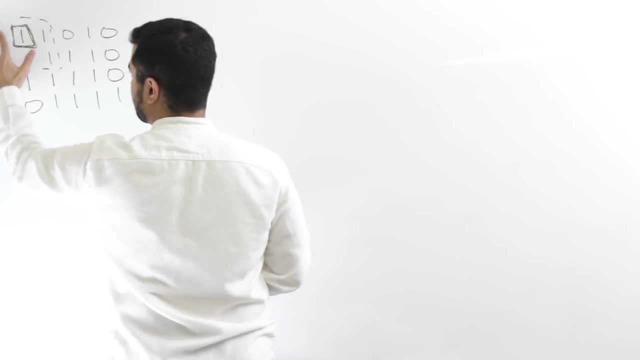 of the of the square right. So, in order for me to get the answer for this particular square- let's say, when I'm, when I'm talking about this one and this is one- then the answer would be: four over here, right, Because that is? or two, sorry, but four ones that make two. 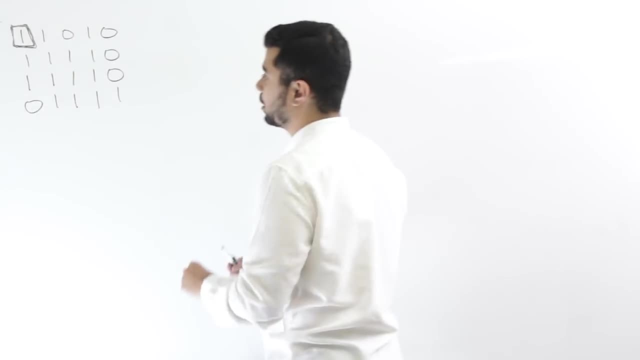 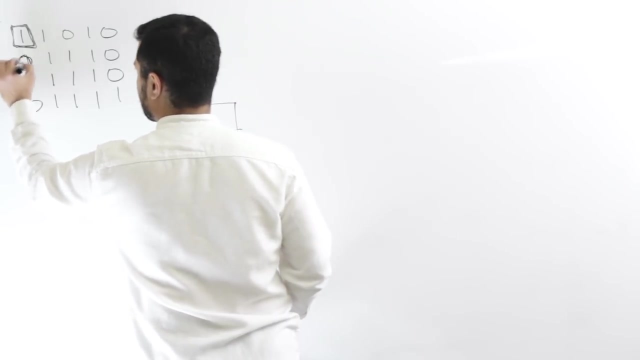 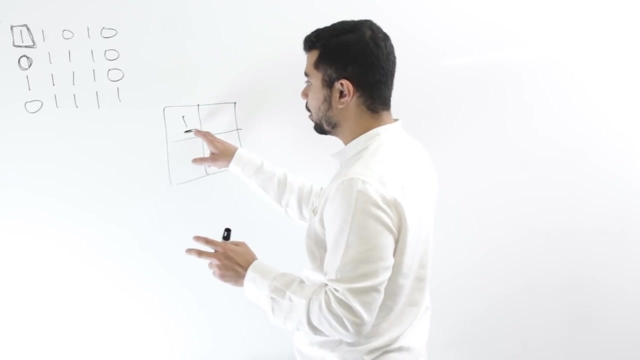 So if I were to go through this logic, then I would say: okay, I have one over here, Let me just make this zero again. I have one over here in order for me to to get the solution for this particular index. And when I say solution for this index, basically: 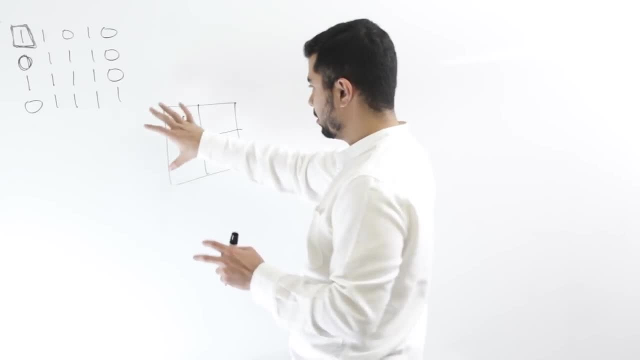 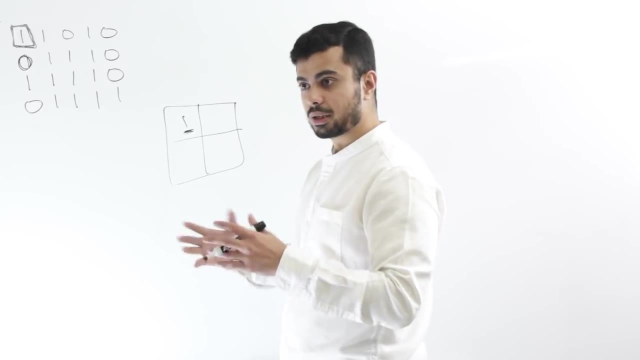 if this index is a top left, like for the square over here, the top left, uh corner of the square, how big of a square it can make such that all of the elements in the square are ones. So it would say, okay, um, let me look at my right, my bottom right, And my, my, my bottom one. 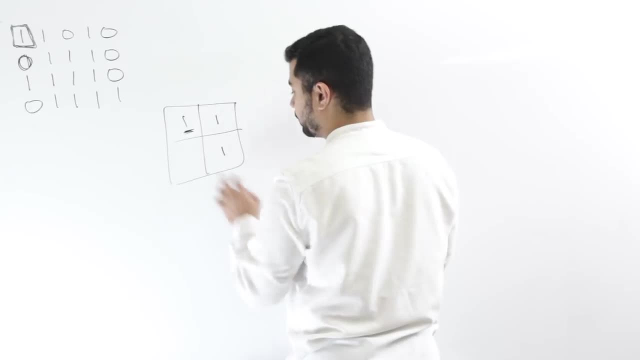 if all of them are ones, let's say this is a one, Okay, Then I would take the. then the answer would be two, right In this case, which is basically: whatever is the value of these three plus itself? right? So one plus itself Now. 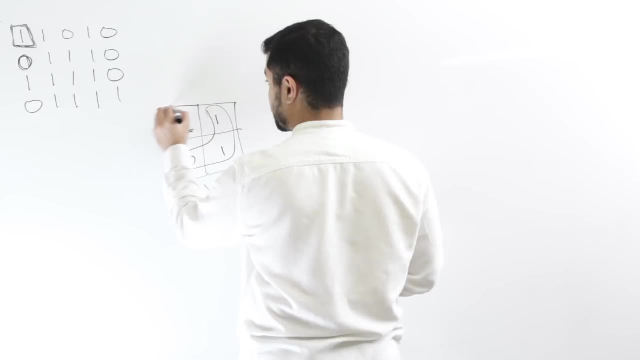 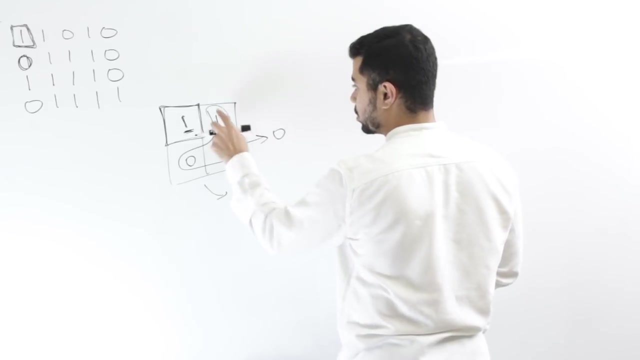 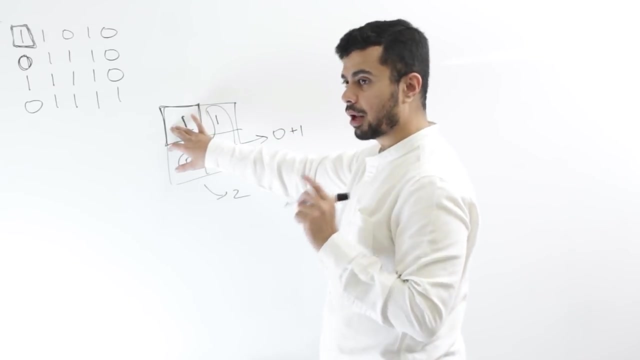 if this was zero, then the value would be one right, Because the maximum square then can make is just itself. So in this case this would be um zero, which is the minimum value of its neighbors Plus itself, right. So any time, then, if we consider this as a top left corner of the square, 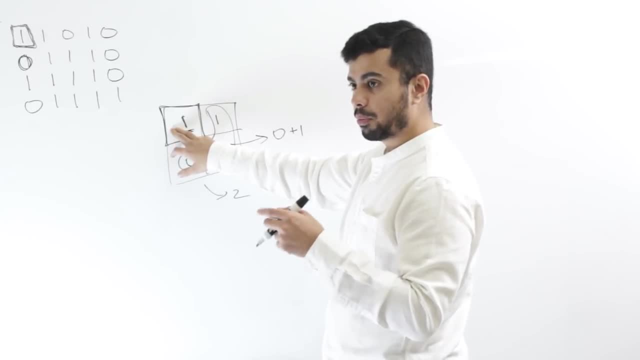 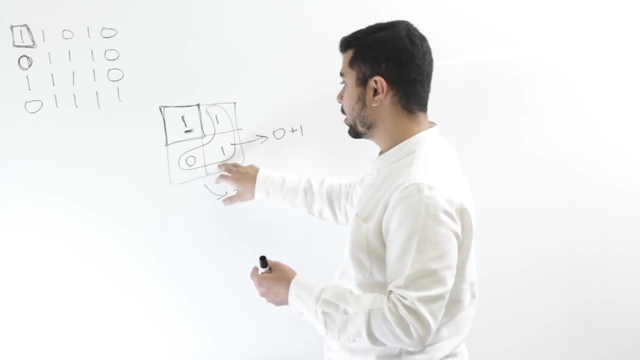 any time I want to check how big of a square of once this can make, then I will need to recurse on these three neighbors to see how big of squares that they can make. Suppose I have the solutions- uh, the recursive solutions- of these three and this one says: okay, I can make. 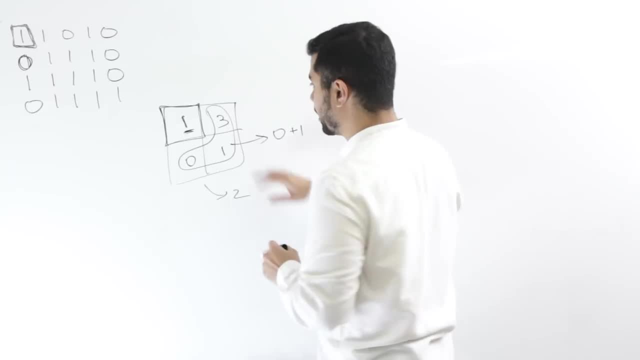 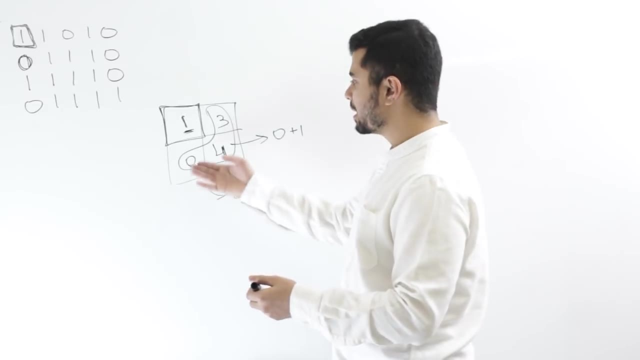 just hypothetically. okay, not related to that matrix, I can make a square of size three. This can say: this says I can make a square of size four, but this still says I can still just make a square of size zero, Like I can't make a square at all. Then the answer would still be: 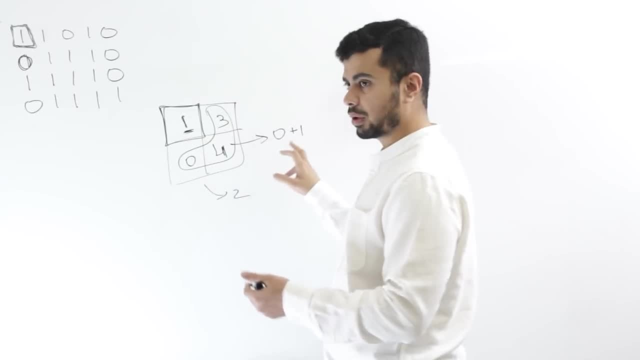 minimum these three, which is zero plus itself, which is one right. And obviously, if this is zero, then this will be zero plus zero, which is zero right. So, um, let's see, um, actually, if this is zero, then I wouldn't even consider it. Okay, Yeah, That is the question. 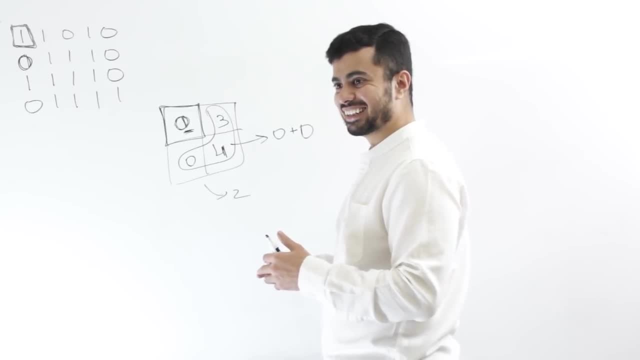 I was going to ask: Okay Yeah, Do you even consider going through all the neighbors if itself is zero? Right, right Yeah, Because if it's zero, then it wouldn't make sense for it to make, uh, a square, right. So let's see how we can, how we can do this over here. 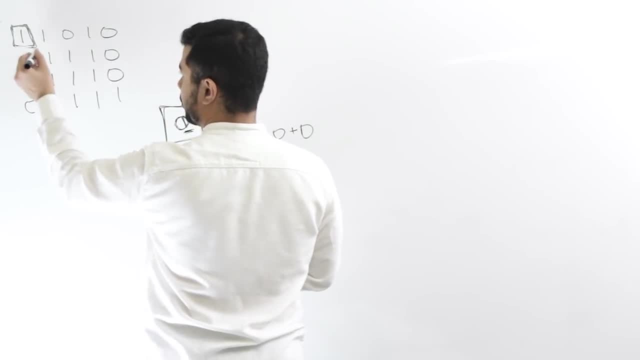 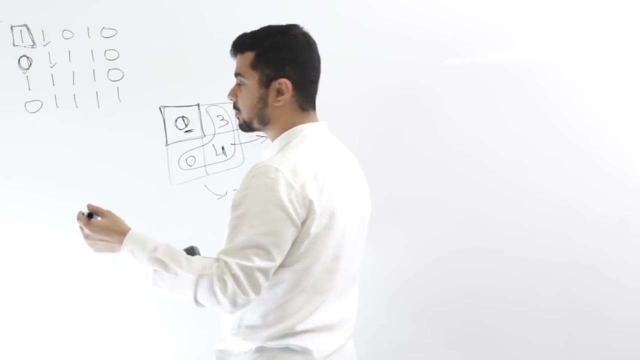 So, as mentioned, in order to compute the value for this particular index, I will need the value of this, this and this Right. So this is a- this is a recursive solution In order for me to compute the value of this one. 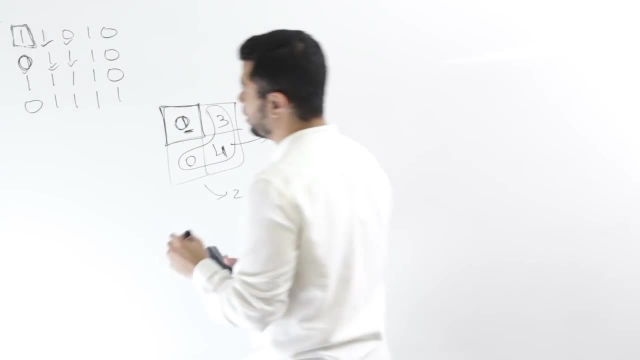 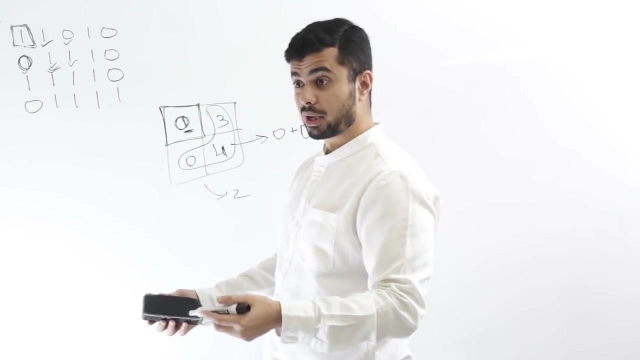 I'll need the value at this, this and this one. Actually, it looks like I'm computing the value at this particular index twice And actually if I want the value at this one, then then I'll have to recompute the value over there, So I'm actually computing it more than. 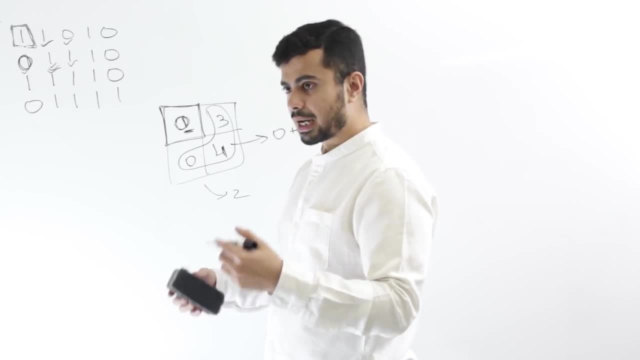 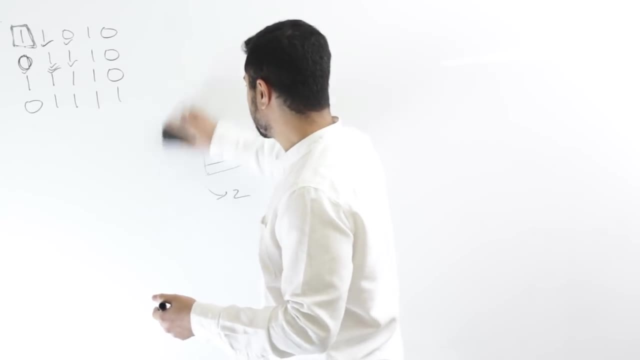 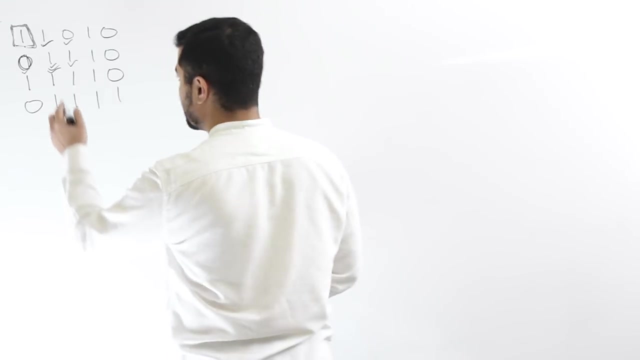 twice, Yeah, So it's not very efficient. So this kind of triggers that perhaps this is a good candidate for for dynamic programming Right. So let me erase this. Let's think about this in a dynamic programming way. Obviously, I'll need some form of cache right for for this, Let's say, as I'm computing this three times: 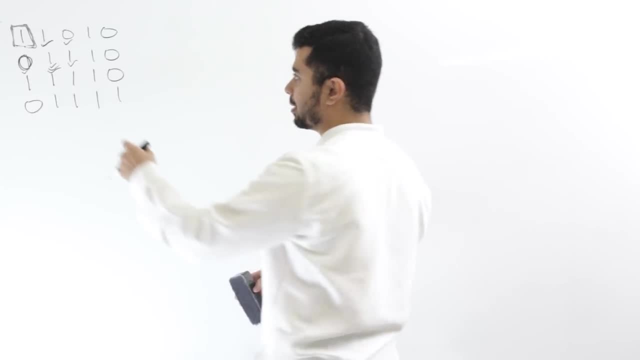 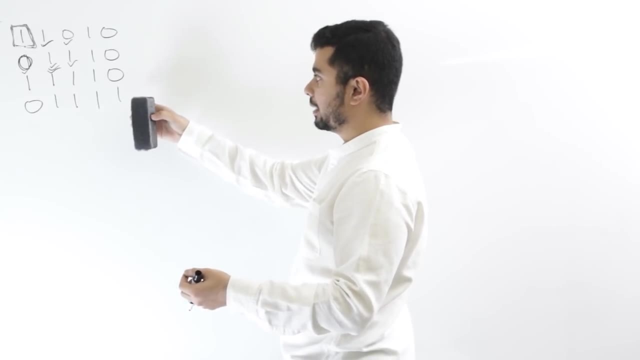 I don't want to do it, so I store it somewhere, And as these values then would be independent for each of these indices, I can just have a matrix of the same length and width, or the row and columns, as this one. 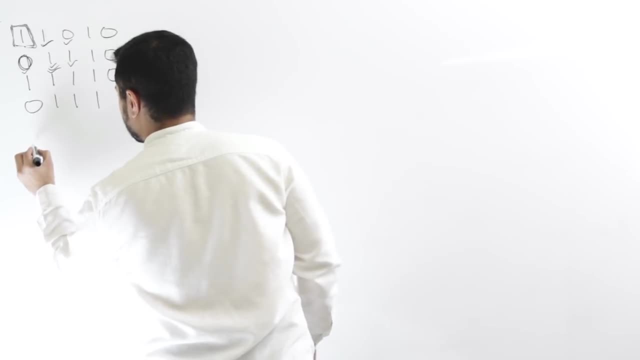 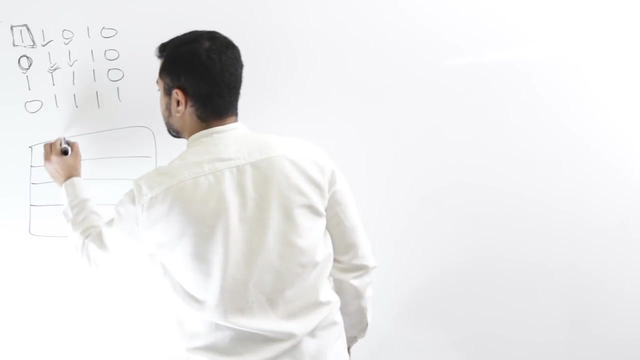 as our cache. So let's say, I have a matrix over here which is 1,, 2, and 3.. And 1,, 2,, 3. Right, And 4, actually there's one more over here, Right. 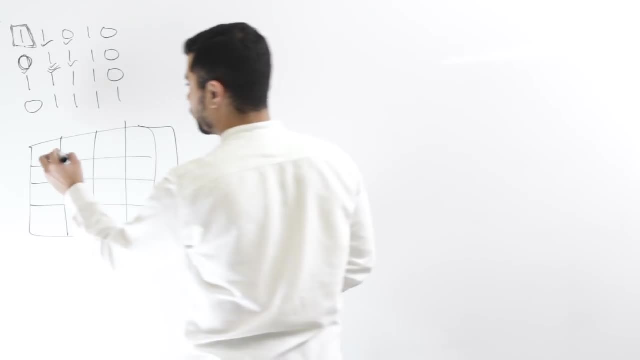 So if this is my cache and I say OK for me to compute the value, Do I need it? 1, 2, 3, 4, 5,. 1, 2, 3, 4, 5 tot mod 3,. can I say OK for me to compute the value? Do I need it?1, 2,, 3,, 4, 5,. 1,, 2,, 3,, 4, 5, 1,, 2,, 3,, 4, 5,. 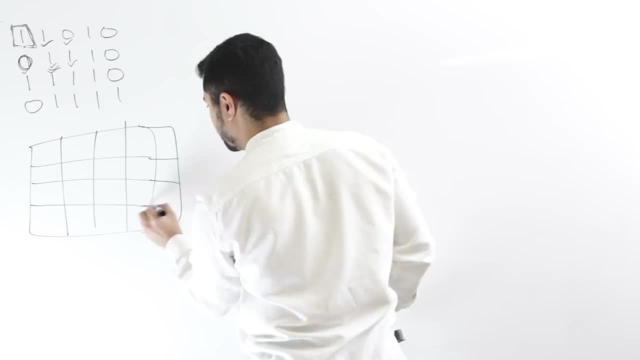 1,, 2,, 3,, 4,, 5, one, two, three, four, five. Yes, I'll need it, Okay. so, in order for me to compute the value for this particular index, I'll say: okay, let me recurse on this one, this one. 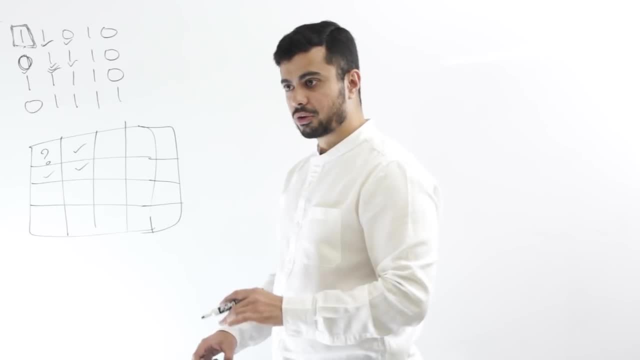 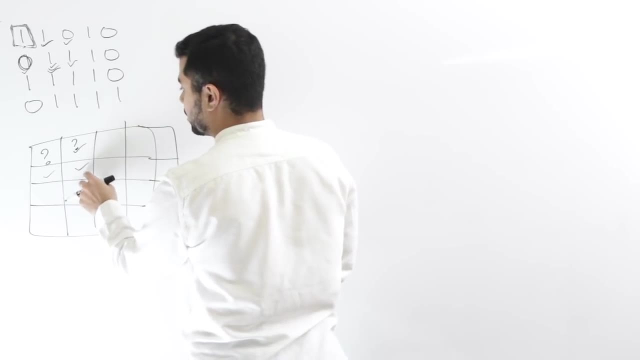 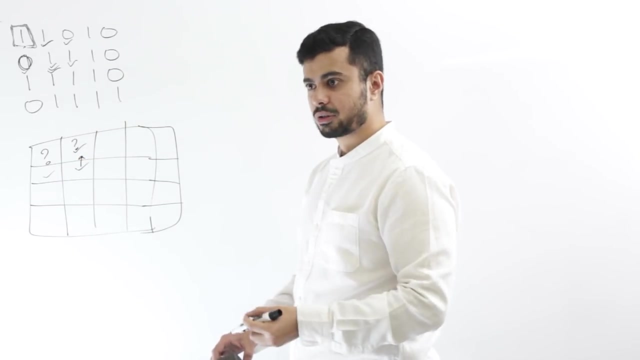 this one and as I'm recursing, let me just save that value in the cache. So next time when I want to compute the value of this, I'm looking at the value over here. I say, oh, I don't need the computation, I'll just return whatever I have in the cache. So I 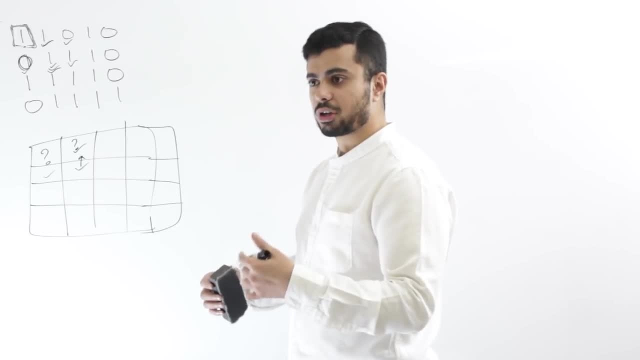 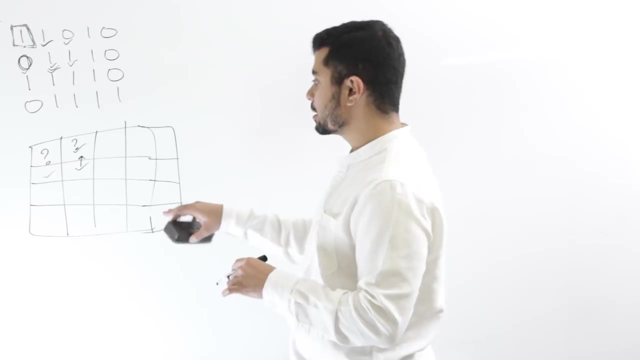 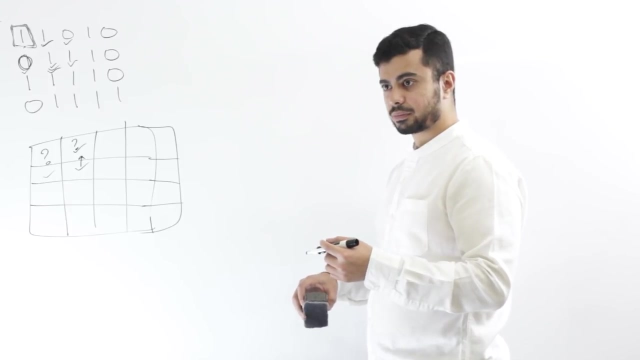 check the cache first and then, if it's not there, then I compute it and then save it right in the cache again, Right? So this is a solution that I'll move forward with. It's a recursive solution, So is this the only way to go around, or can you make it iterative? 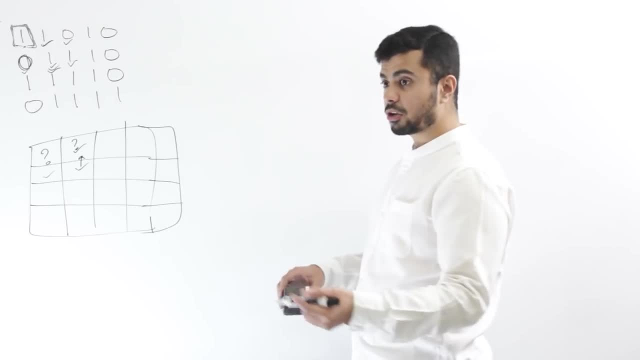 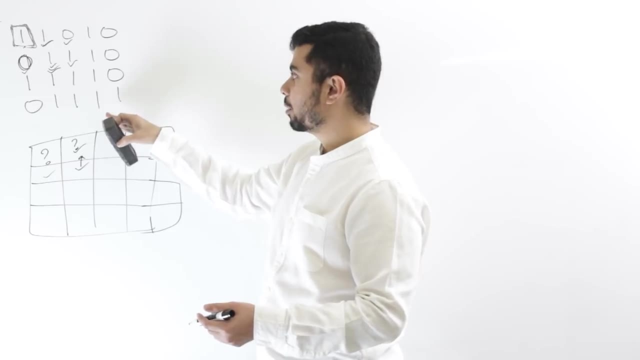 Can I make it iterative? I can make it iterative. I can make it iterative as well, actually. So I will just need to iterate through all of these squares, all of these indices, and compute their own values. But obviously, now, as I'm iterating through them, I will ideally want to leverage the values that I've already. 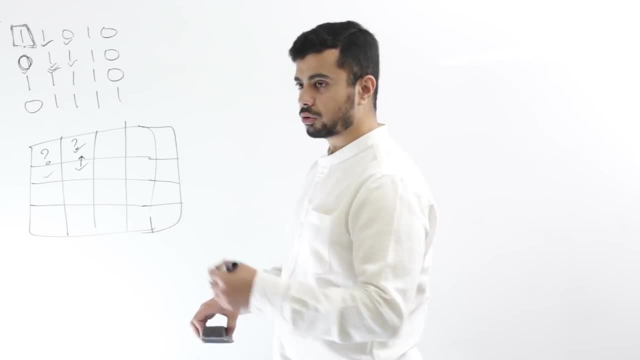 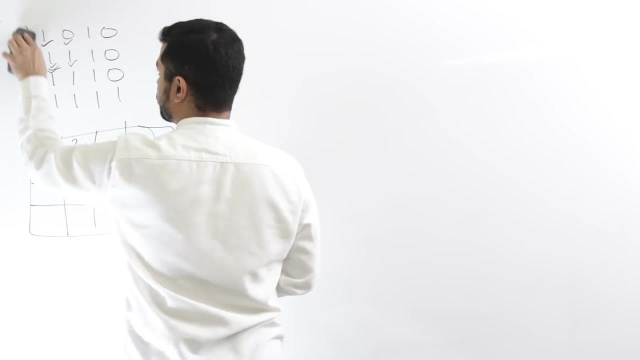 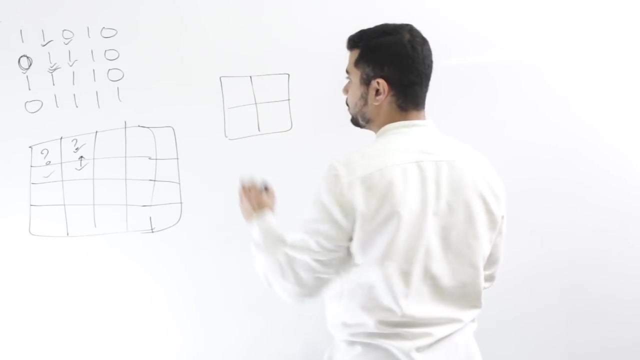 computed to come up with its solution. So actually, then, if I'm iterating, I should consider each one of these indices not as a top left but as the bottom right. So right now I was saying okay for this particular answer. I need the answer to this, this and this. 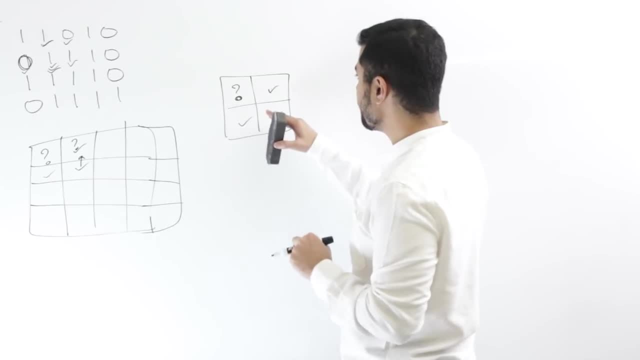 one, right, Yeah? Now if I'm iterating, I'm going from zero to whatever is a length minus one When I'm at this particular index. I don't really have the computation for these three yet, right? Yep, So I can say: okay, instead of me counting the index as the top left corner, let me regard. 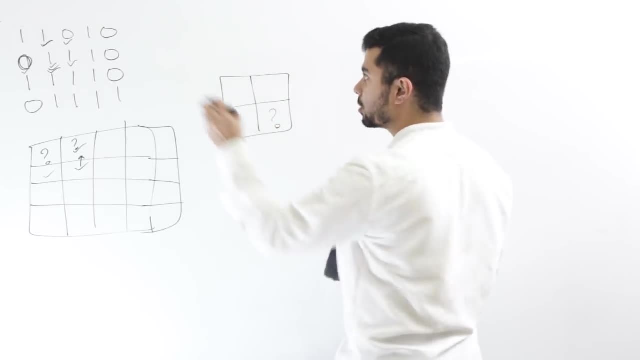 it as the bottom right corner. So if this index is the start, is the top left of our matrix itself, then I start over there. And as I'm at the top left, and that is the bottom right of our matrix, of our square, or the maximum square it can make, then the answer is just itself. 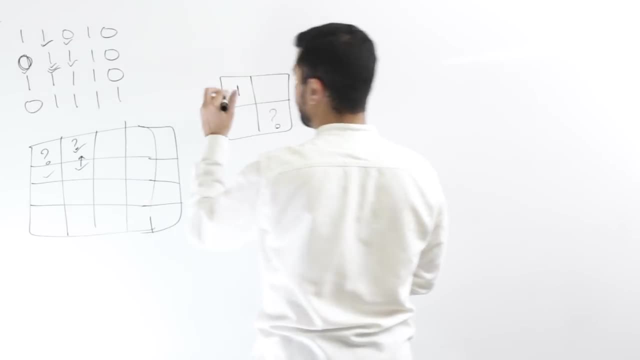 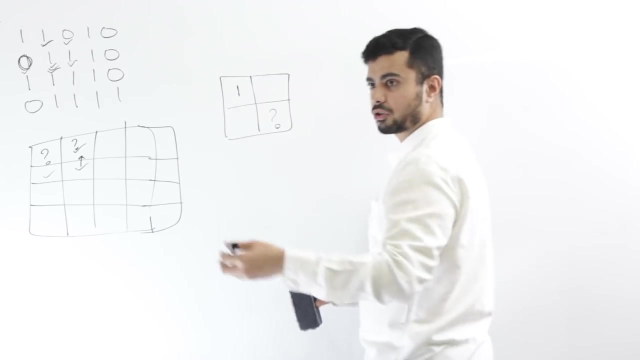 Then this will be 1. Same thing over here. So I think the leftmost column and the topmost row, the answers for those will be just itself, Considering they are the bottom right corner. Considering they are the bottom right corners, yes, of the square. 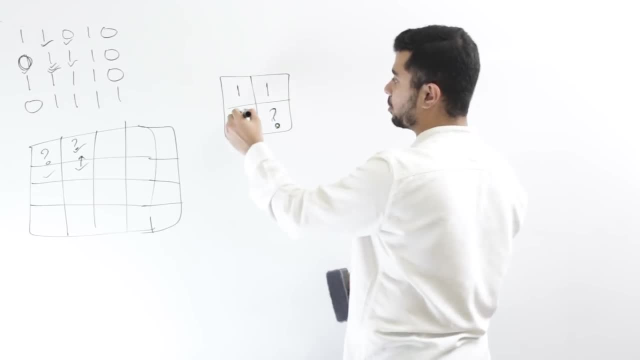 So I'll have 0 over here, And then, when I'm here, I know the answers to these three neighbors- I can say: okay, in order for me to compute my value, I need the minimum value of these three. so now the logic is the same: I'll need the minimum value of these. 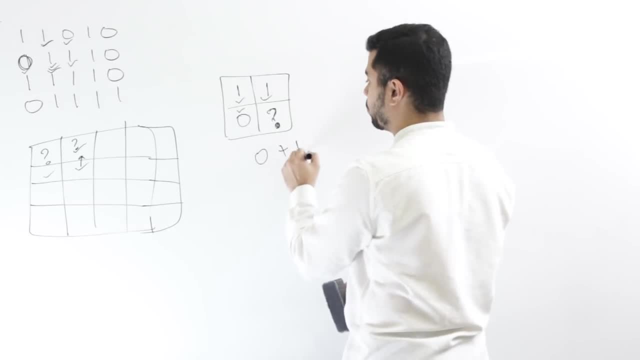 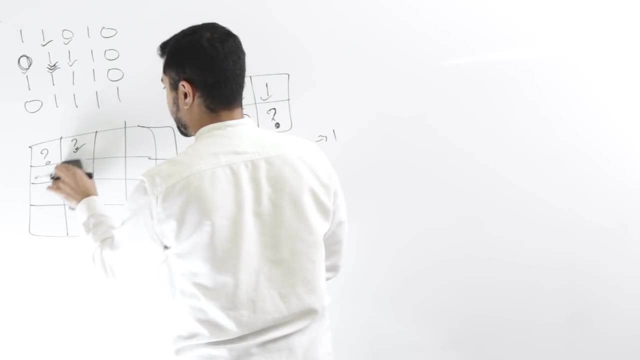 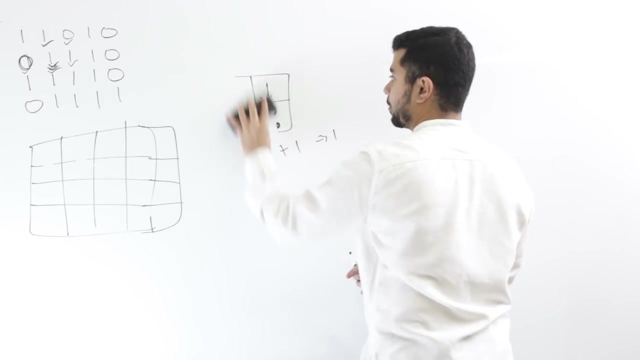 three plus the value of myself. so it'll be 0 plus 1, which is 1, right? So the answer for this particular index will be 1.. So let me just erase this Minimum of all its neighbors plus itself, Right? 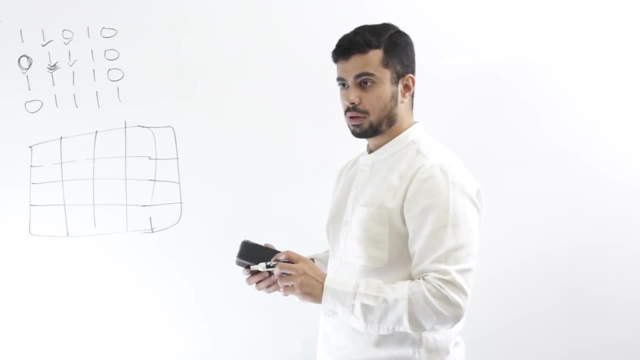 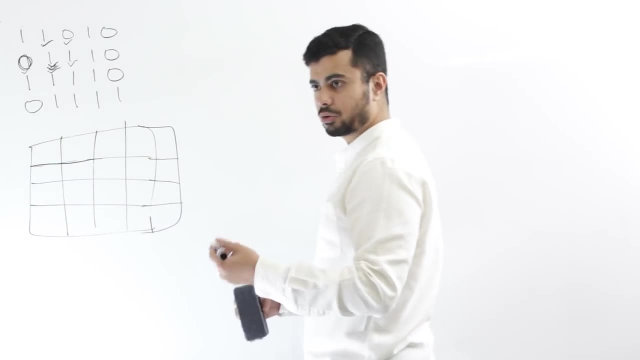 But if it is 0, do I still do the same? No, if it's 0, then I wouldn't go through the computation. So let me just go through an example over here and then I'll go through the actual implementation. 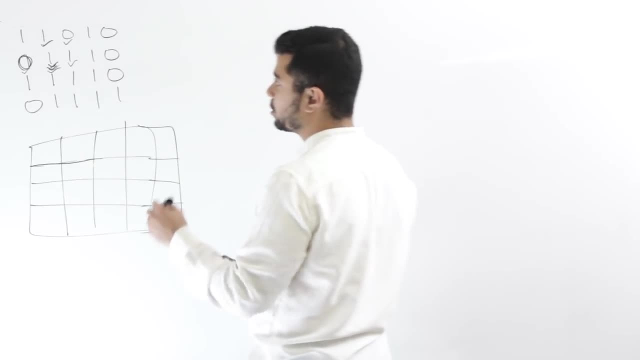 if that's okay. So I start. let's say i equals 0, and then so i is the row, and then I'm just iterating through all of the columns: So i equals 0, and j equals 0 right now. So I'm over here. 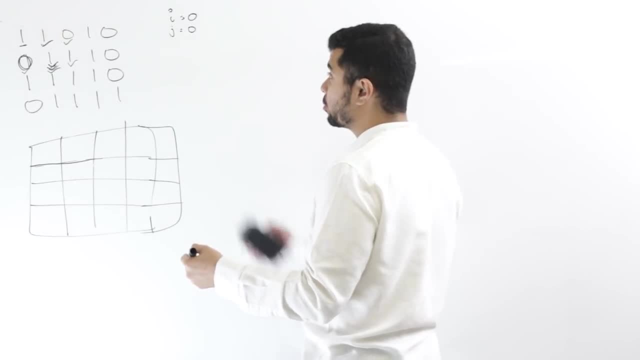 And I say, okay, what is what is actually when i equals 0 and j equals 0,, then it is just itself, Right, I don't need to do anything. If either one of these indices is 0,, then 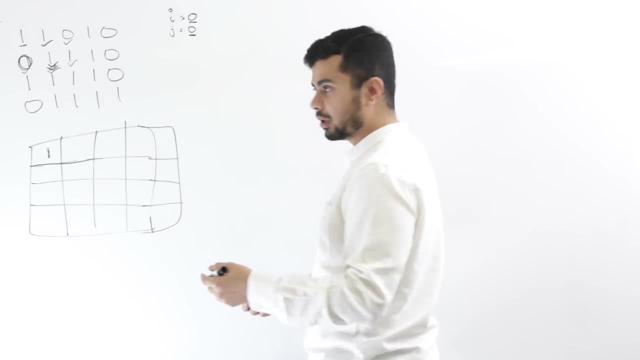 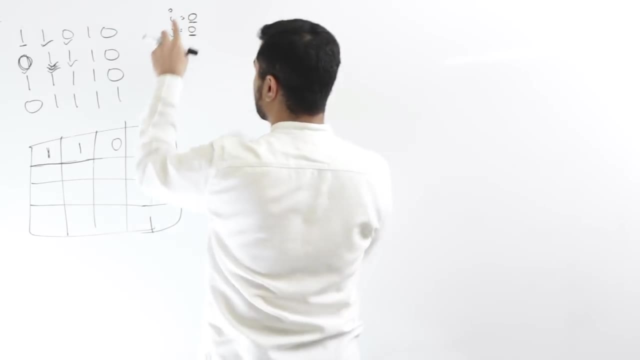 the answer for the maximum square will just be itself. So I say, okay, this is 1,, this is 0,, this one is 0,. right Now, I'm in the second row, so now Can you go through one of them? 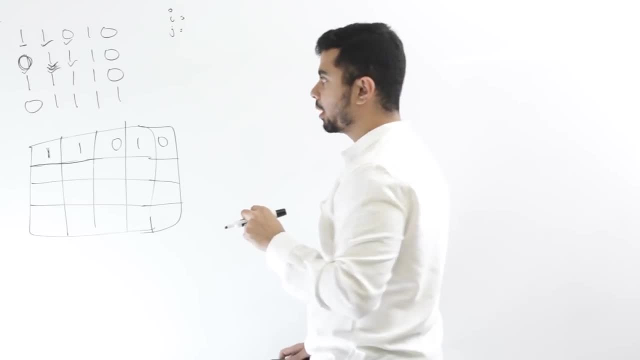 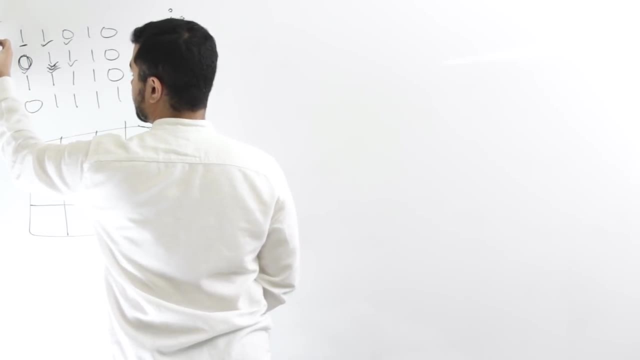 Sorry, Like why the answer will be itself. Why the answer will be itself. So if this is the bottom right corner, then I'm looking at its neighbors- Neighbor over here, neighbor over here, neighbor over here- but these three fall outside of the matrix, right? They don't exist. 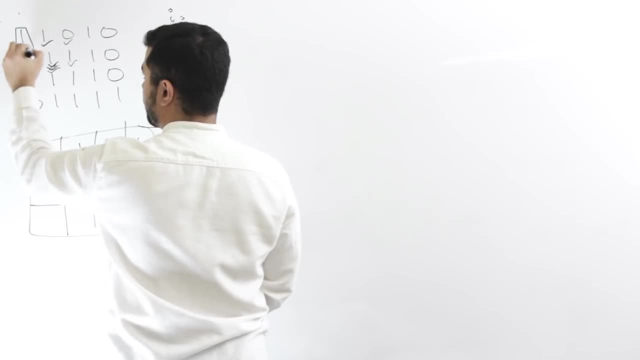 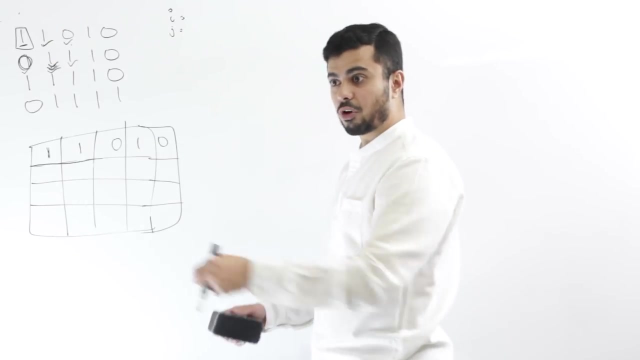 So the maximum it can make is just itself: Okay, If I'm over here, then same thing. one of the neighbors is falling outside. So anytime one of the neighbors fall outside of the matrix, then the answer will be just itself, Because the minimum will be 0. 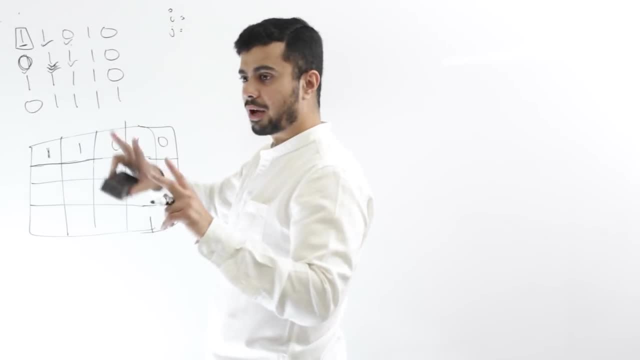 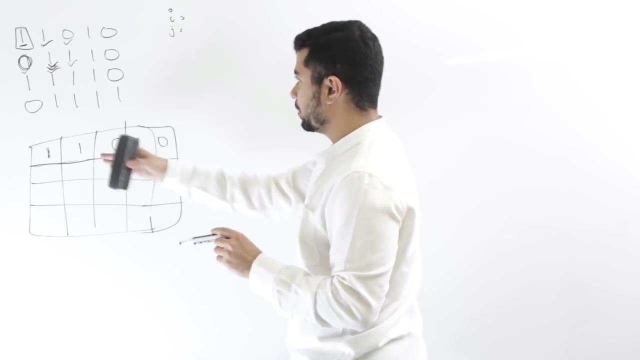 Because the minimum will be 0,. yeah, Anytime the neighbor is outside, then that value is 0.. Yeah, That makes sense. Okay, So in this case, now I have all of these values right, Then this for when i equals 1 and j equals 0,. 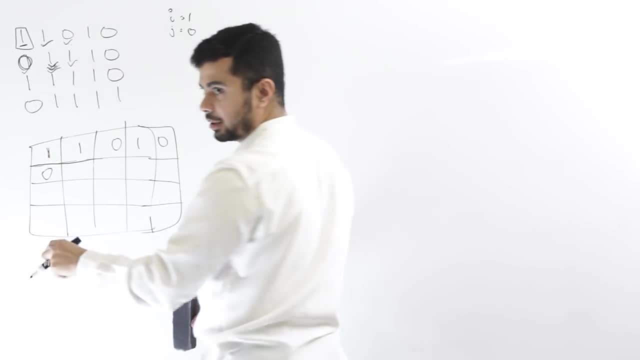 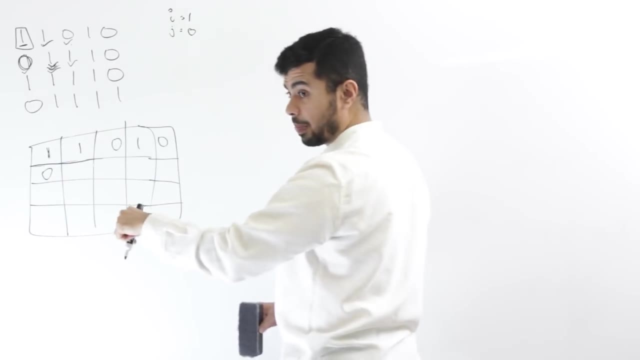 still one of its neighbors is outside. So that is itself. Now I'm at 1, right, I see? okay, I already have these three computed. So I take the minimum of these three and I add 1 to it, So this will be. 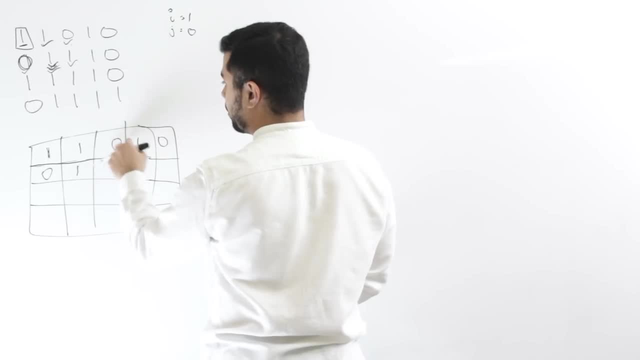 1, because minimum is 0, right, And then I go over here: the minimum of these three: I add 1 to it. I go here this for this one same thing: minimum of these three, I add 1 to it. 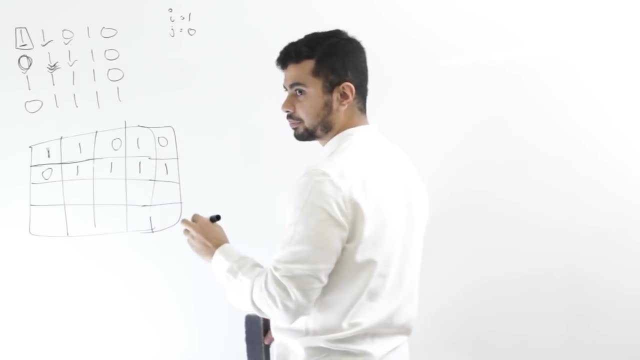 Same thing over here. I add 1 to it. right, Add 1 to it. Sorry, this is 0, so I don't even compute it. Good catch, I wasn't even looking at the matrix. Okay, Now I'm back over here. Now, j equals. 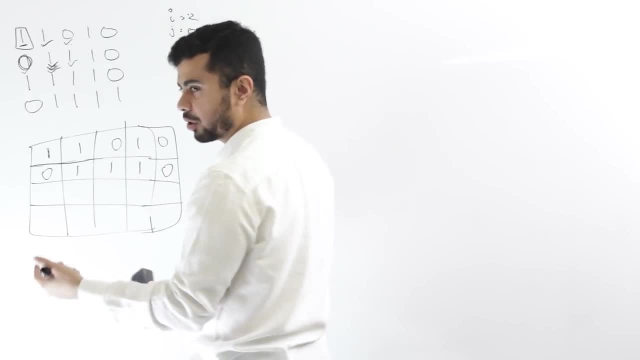 now i equals 2 and j equals 0 again, right? So anytime j equals 0 or i equals 0, it's just itself. So I add 1 over here. Same thing for this one. I'm computing it as it's 1,. 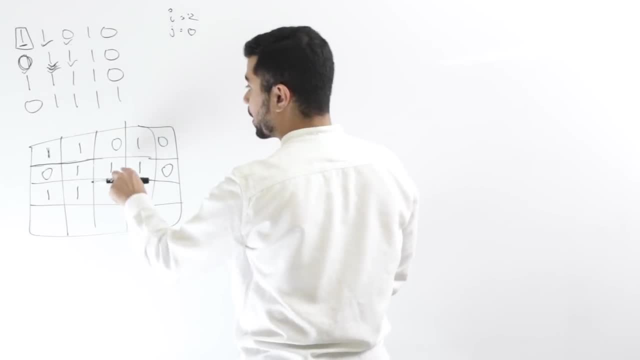 and this neighbor is 0, this will be 1, right, But for this now, it will be the minimum of these three, which is 1, and then this guy is 1 as well, so this will be 2.. 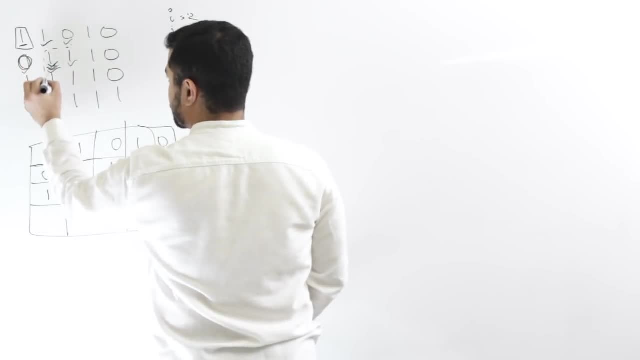 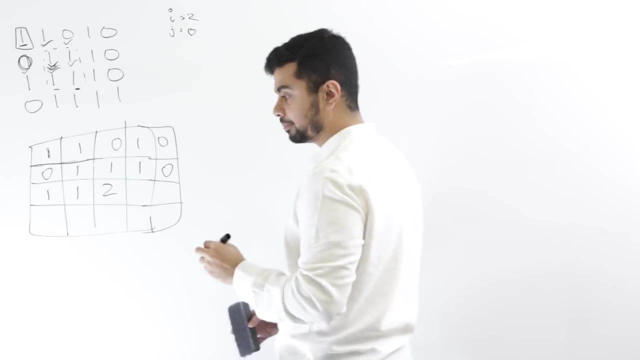 Yeah, So, because I'm making this square over here- of side 2.. Considering this as the bottom right corner. Considering this as the bottom right corner? yes, Makes sense. yeah, Now, as I progress forward, I'm here, right. 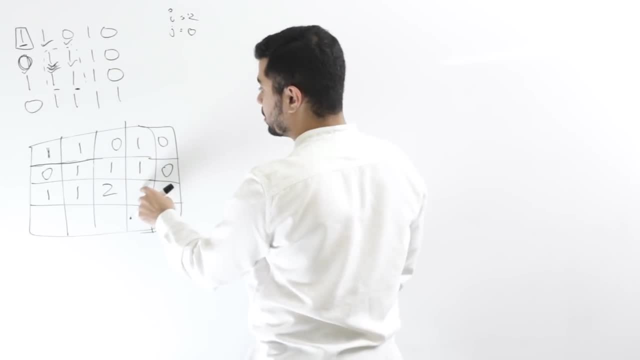 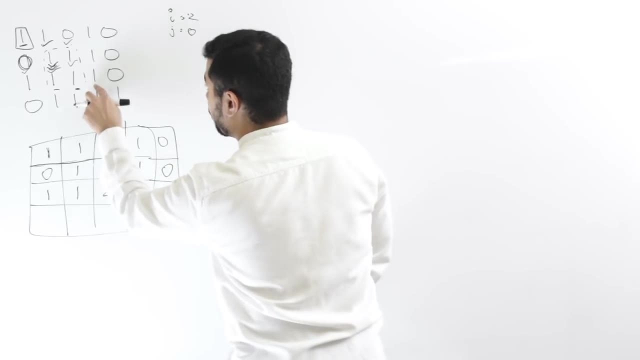 And I look at, okay, it's neighbors And this is 1 as well. So the minimum over here is still 1.. So I'll just have 1.. 1 plus 1 is 2, right Yeah, So this will make this square, right here. 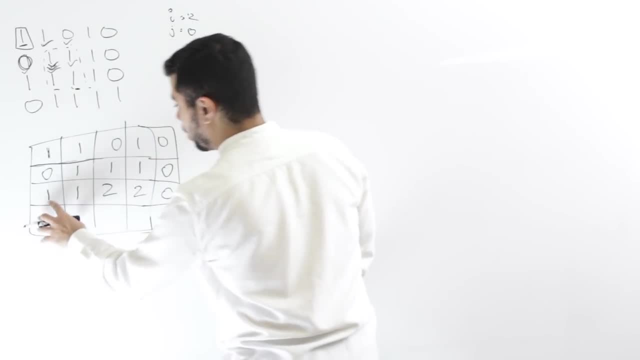 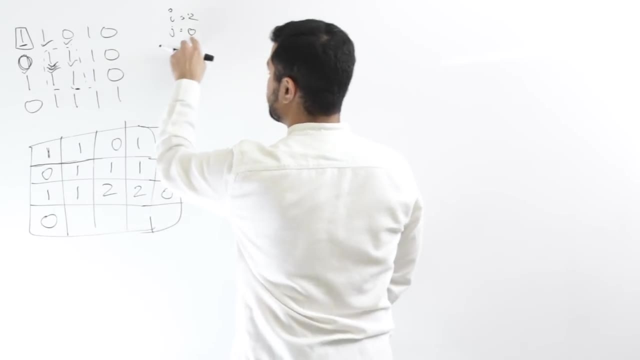 We add 0,, so I won't do anything. And for all these bottom ones, for all these bottom ones, I have 0 over there, because j is equal to 0.. This will be 3,, right? And for all of these, I'll just. 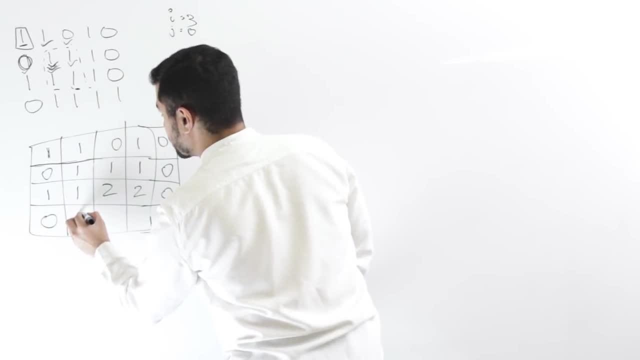 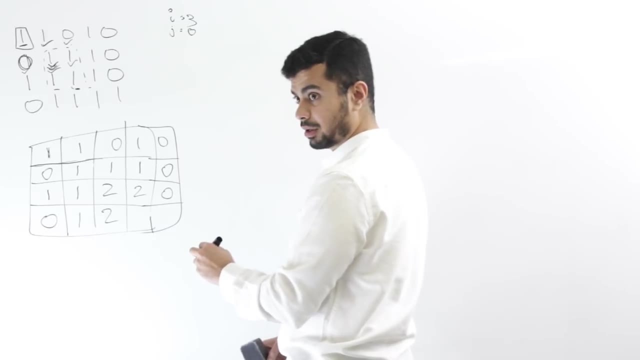 do the same thing again. So 0, 1, 1.. So this will be 1.. 1, 1, 2.. So this will be 2.. For this one, it's 2, 2, 2, actually, Right, So it'll be 2.. 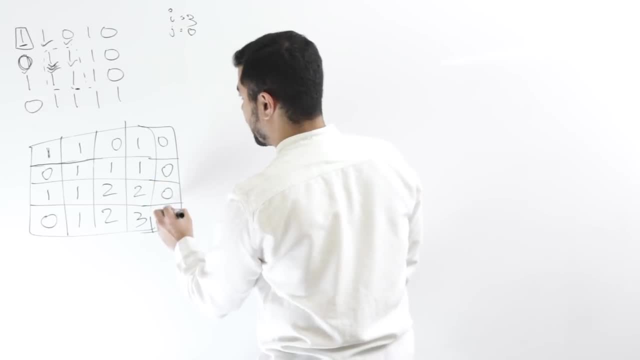 Minimum is 2 plus 1.. So this will be 3.. And the last one is going to be 0 plus 1.. So it's itself. So in this case, our max value is the value right there. So, actually, as we're iterating through it, 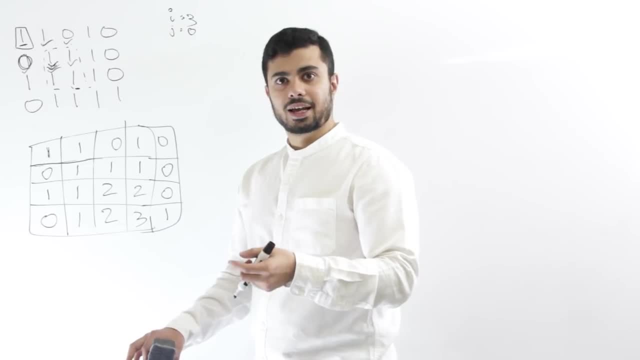 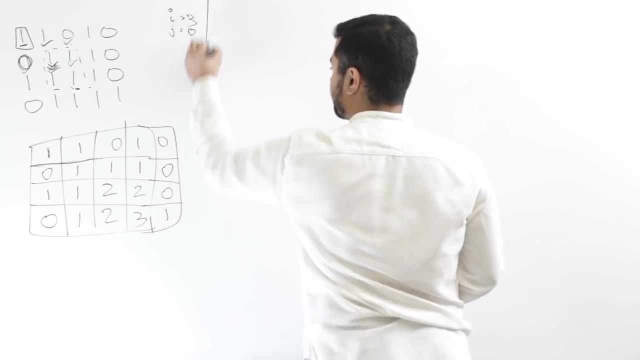 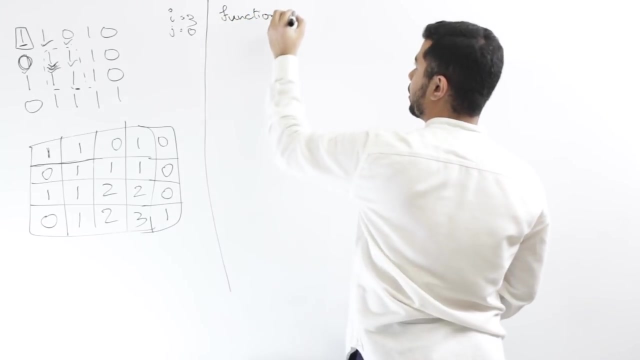 we can also keep track of the max as we're going through the iterations And at the end we just return that value. So let me now go into the implementation. Yeah, sure, Let's say I have a function And I say the name is largest. 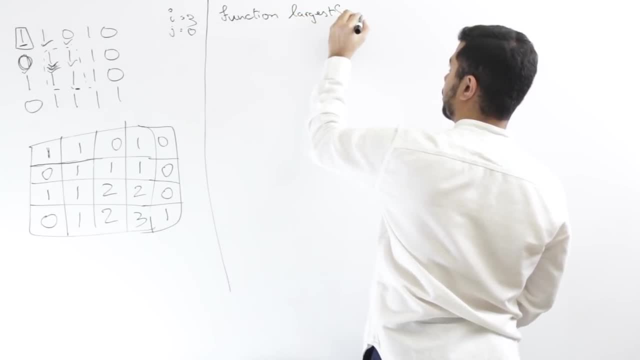 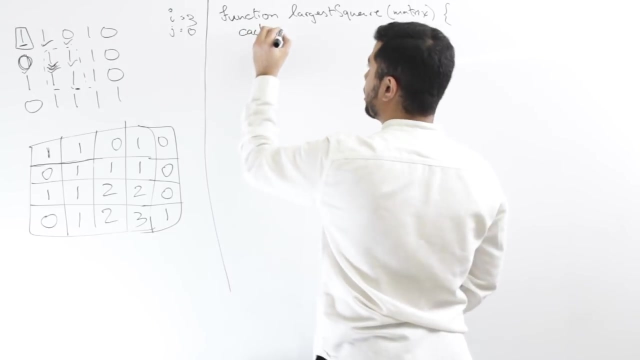 square. It takes in a matrix. Right Now, the first thing I need to do is form a cache. So let me do that. Let's say cache. So this is a pseudocode. Cache equals an array. Let's say: 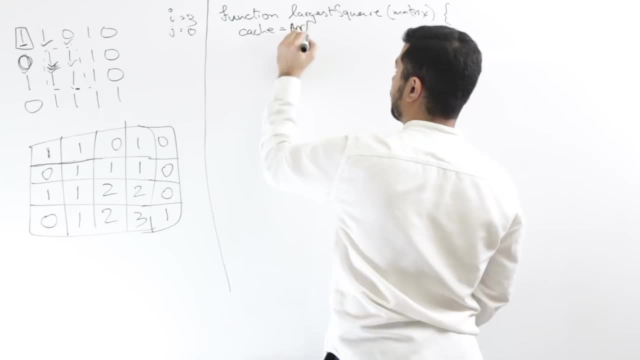 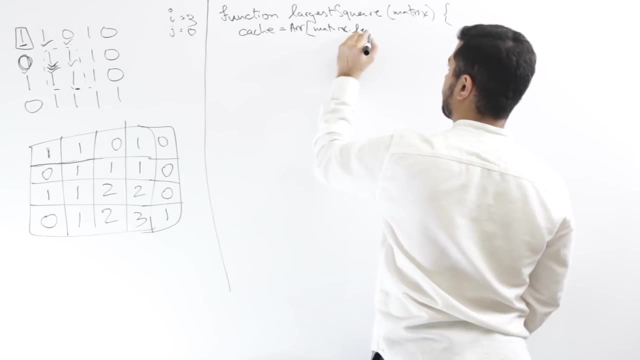 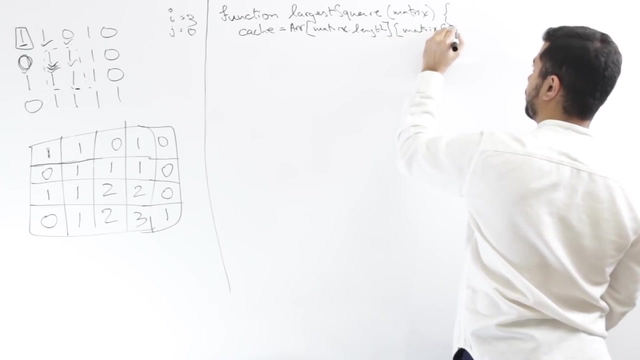 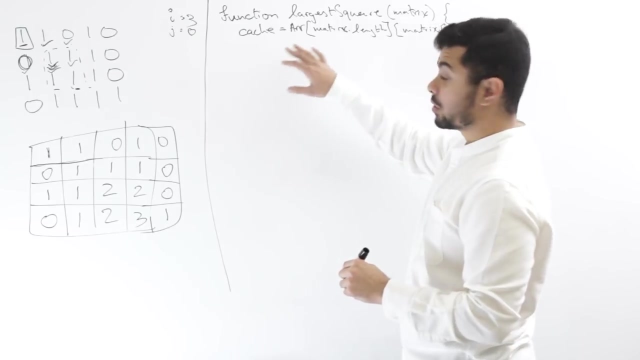 an array of length, matrix dot length. And it's an array of arrays, right. So matrix 0. dot length, Alright. So actually, if this was JavaScript, I would actually have a for loop and go through populating the values inside of the 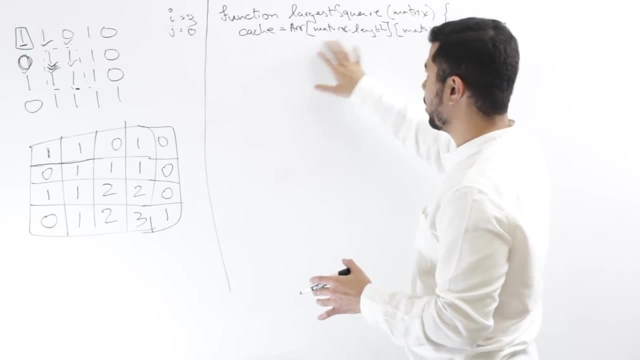 cache just to make sure that it's particular length, But for now pseudocode. let's say this is basically a clone of the matrix itself. Yeah, So let's say we are now also initializing max, So max or. 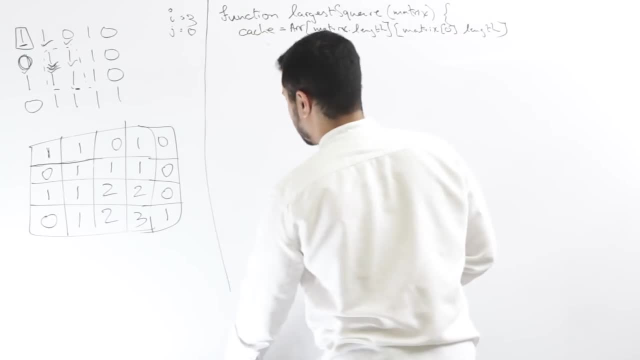 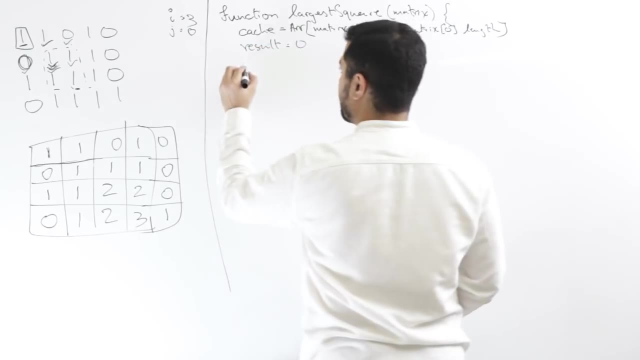 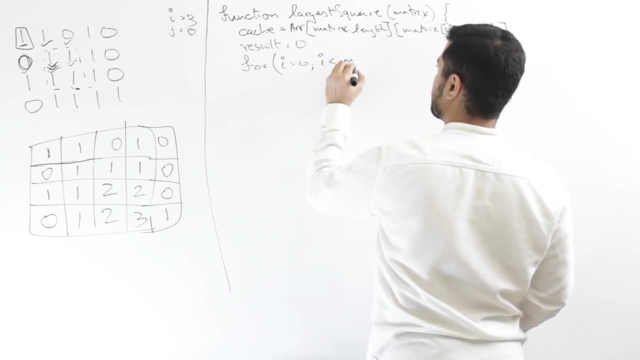 let's just call it result, right, Because it's going to be result that we return at the end. Result equals 0 initially, And then I go into a for loop: i equals 0.. i is less than say matrix. 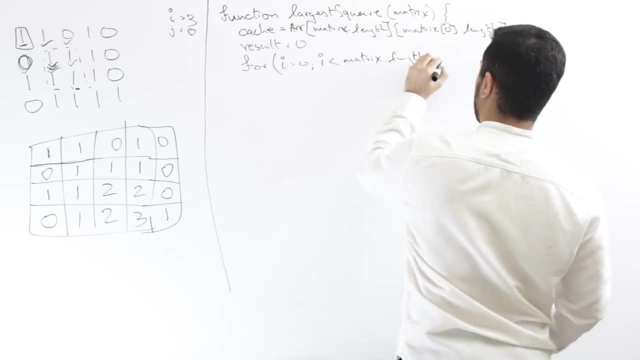 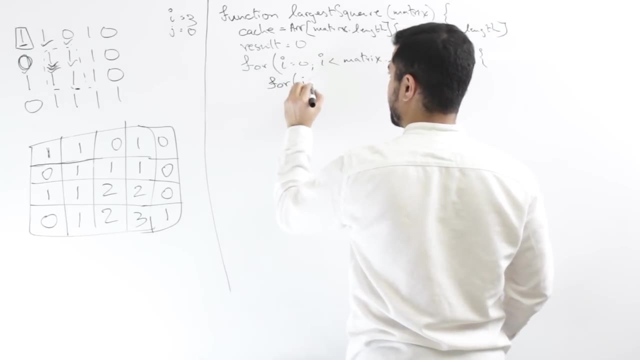 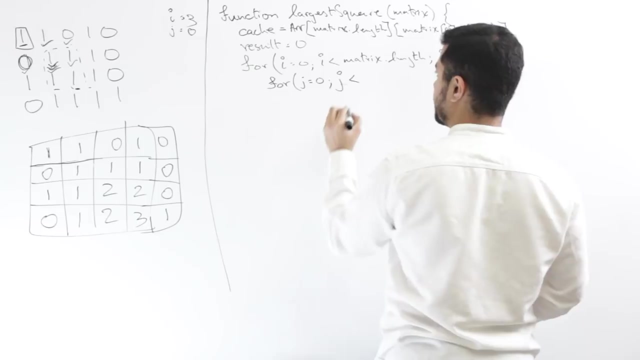 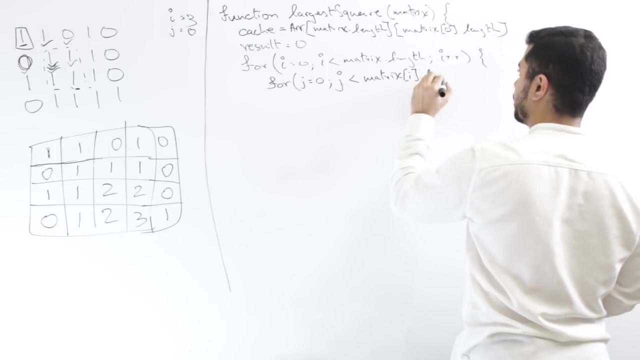 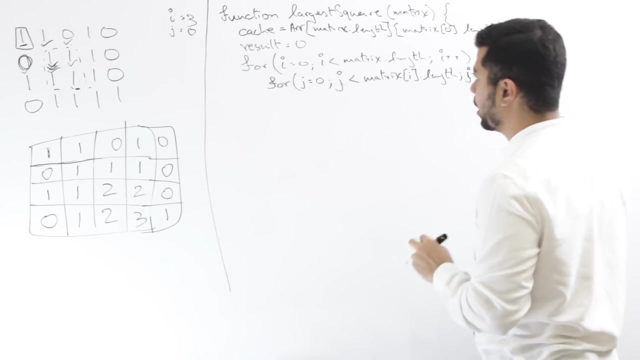 dot length And i plus plus Yeah. And then I have an inner for loop: j equals 0. j, j is less than matrix i dot length And j plus plus Yeah. Okay. So now what do I do? The first thing I do is I check whether or not. 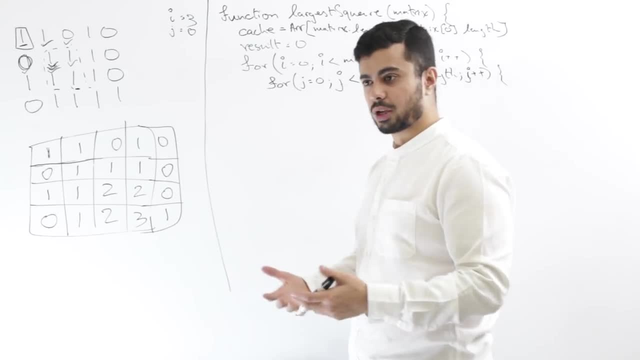 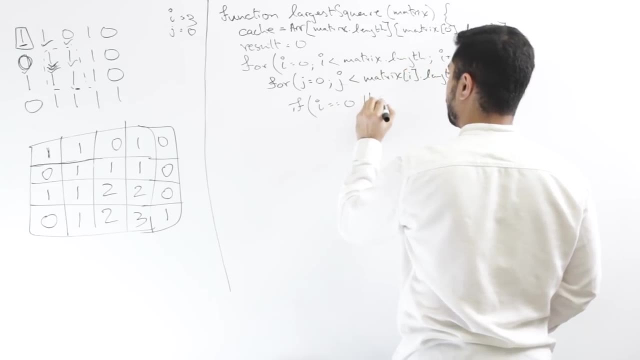 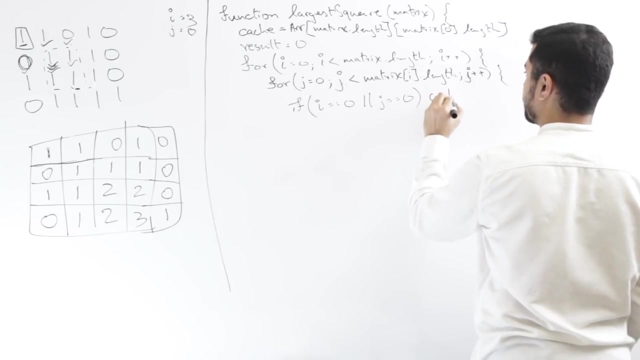 either i or j is 0. If they are 0,, then I don't do anything. So I say, if i equals to 0, or j equals to 0,, then I say cache i j. So ideally I would actually. 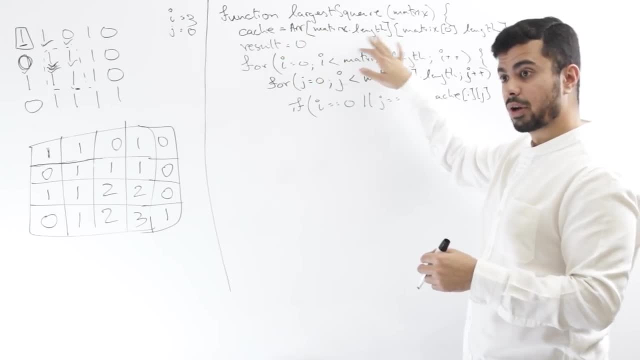 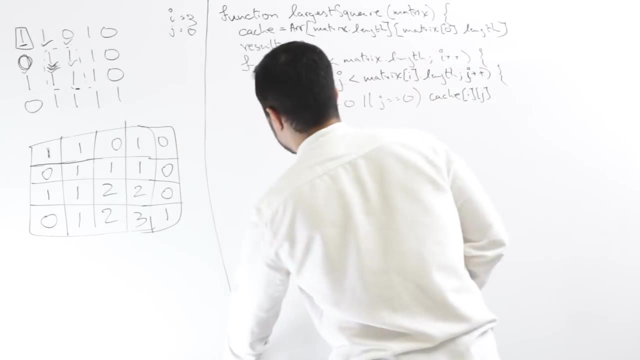 clone. I would have the cache as a clone of the array itself, Because as we are iterating down, we are sure that we are modifying the value, So it won't really matter. So let me just simplify this a little bit. 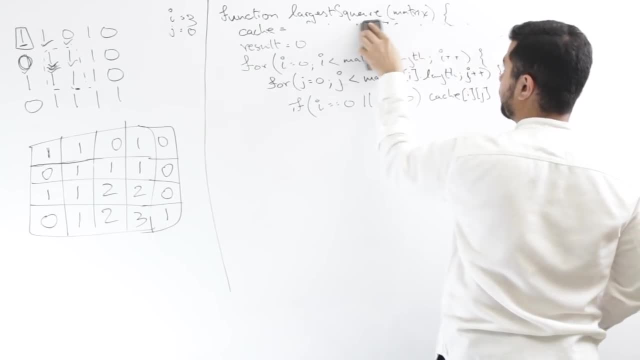 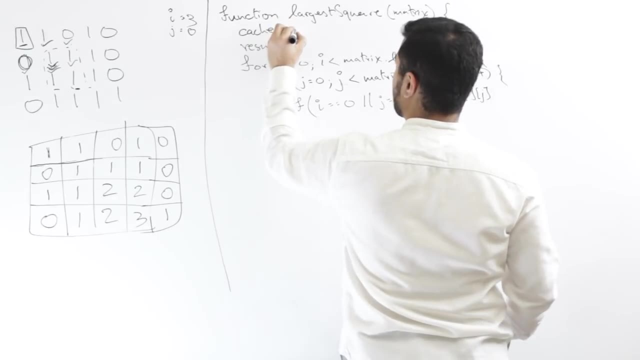 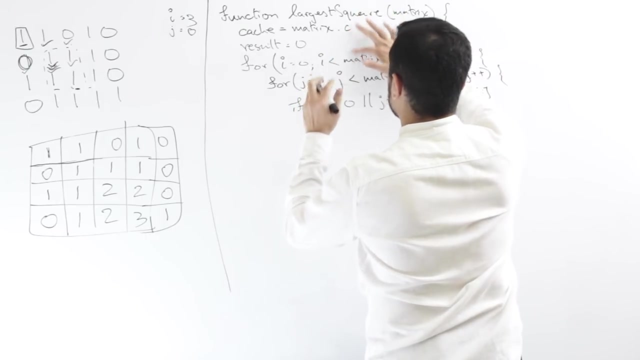 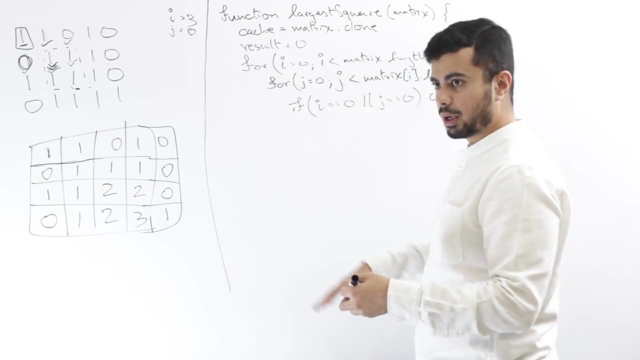 Okay, I'll say this is just a clone of the array Or the clone of the matrix. So I'll say matrix dot clone. So if it was JavaScript, you would basically be populating it with the same value, Exactly. yeah, I'll have a for loop and I'll populate the new one with the same. 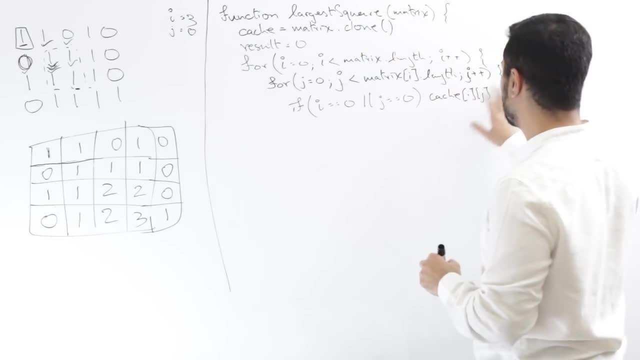 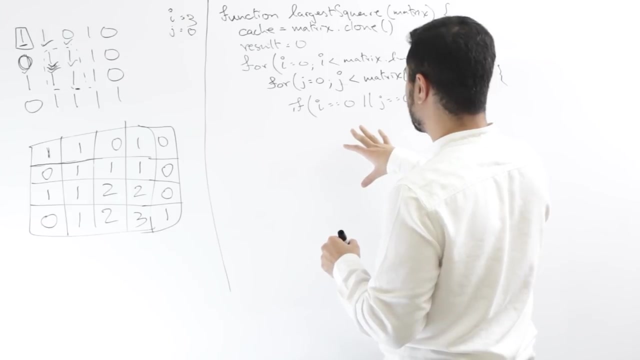 values. So I have matrix dot clone. So in this case, now if this is the condition and it's met, then I won't do anything, right, Okay Now? the second condition would be that now we have to check. okay, if this is. 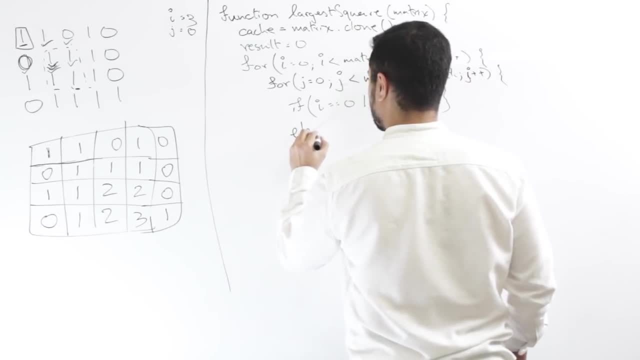 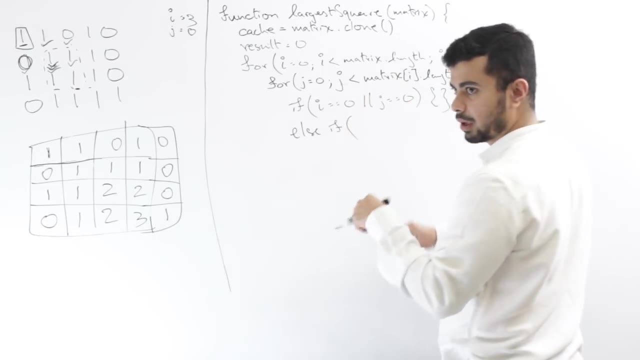 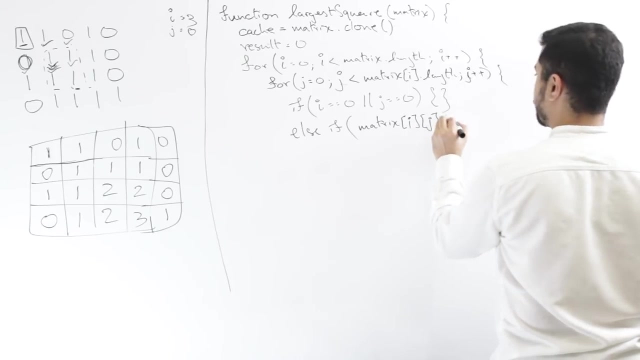 not the case, then what do we do? So we say else, if i or the value itself is not zero, then we do something right. So I say: if matrix i, j is greater than zero, Basically it's not zero or it's one. 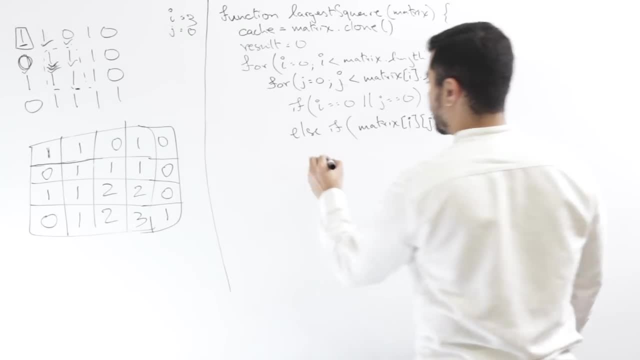 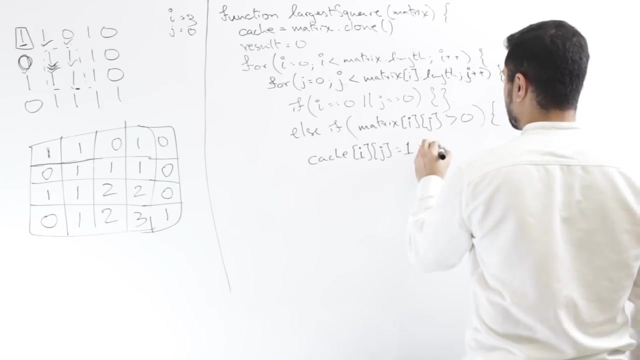 Then what do we do? We say: cache i j equals. we said: we add one to whatever it is right, Because we know it's not zero anyways. We add one to the minimum value of its neighbors. So let me say min. 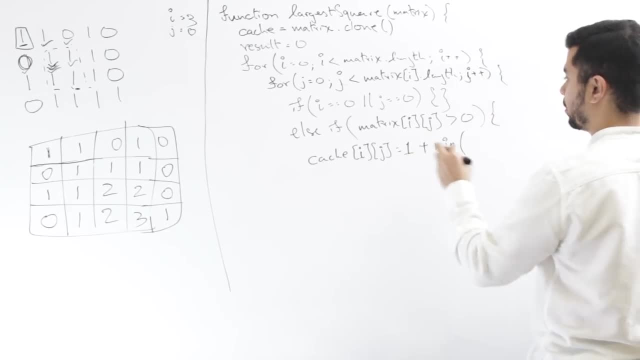 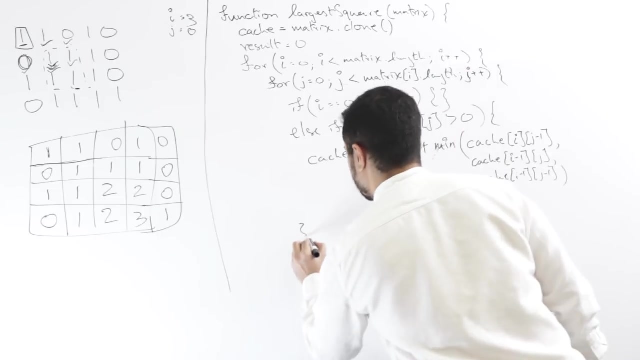 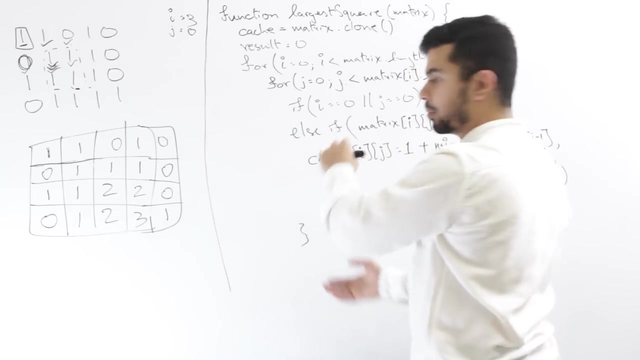 min. of cache i j minus one. cache i minus one j and cache i minus one, j minus one. Right, Yeah, So this looks good. Now I will close that statement and at the end I will modify my result. So I'll say if So, this is still inside of the for loop, I'll say if: 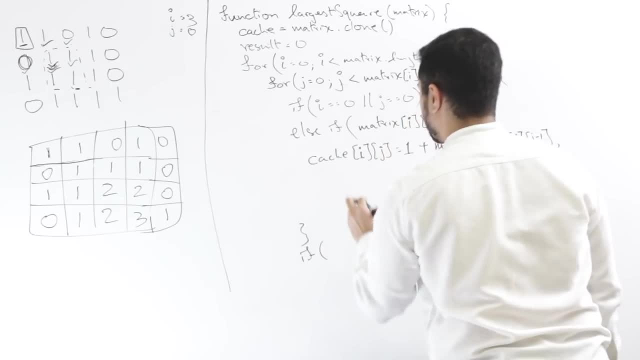 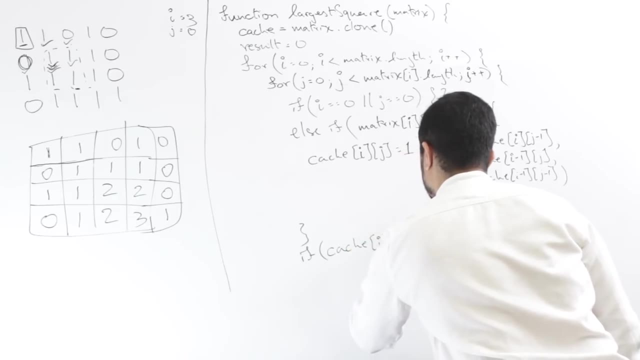 if result or if cache i j- let's say i j- is greater than result, than result equals cache i j. Yeah, Yes, And this will close our for loops And after the for loops, actually I'll just return the result and I'm done. 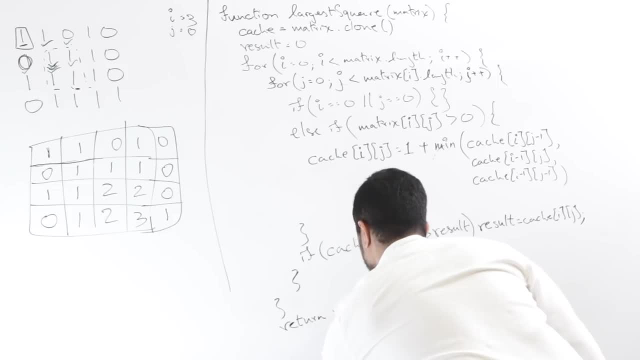 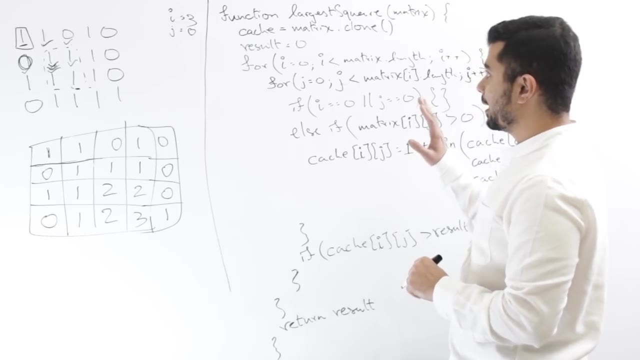 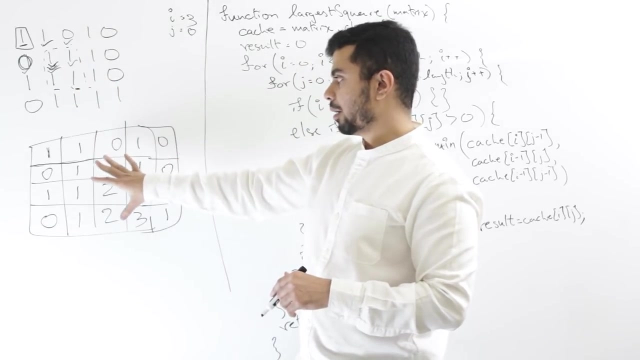 So return result: and that's it. Yeah, that's smart, Yeah. So in order for us to kind of increase the efficiency and not compute things three times, we had to allocate some space right. So we're compromising space. 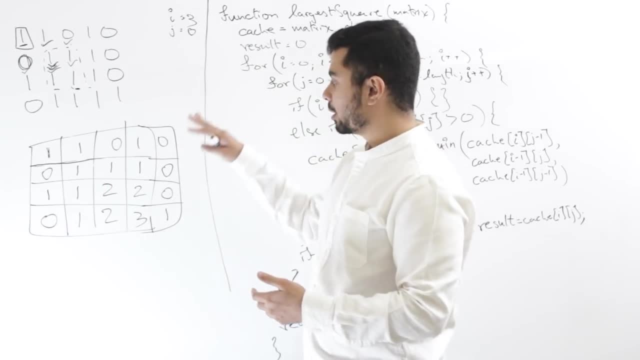 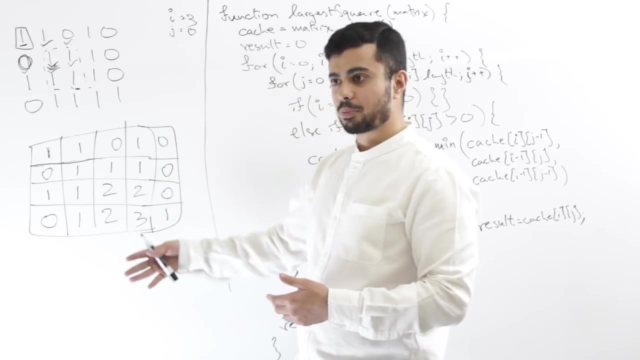 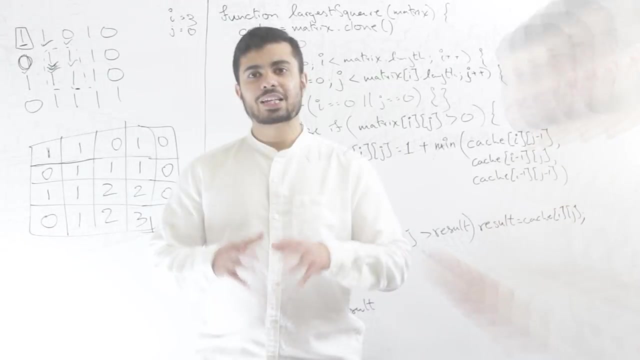 for optimized time complexity, But essentially we'll have a n by n or n by m- space complexity as well as time complexity. Yeah, because you're, just Because I have a nested loop. Yep, Thanks for watching, guys. Today's video was an excerpt. 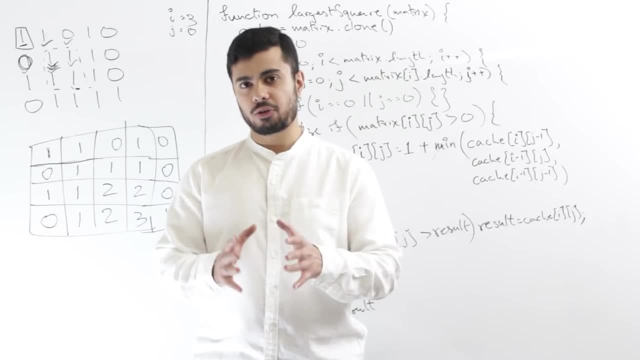 from a data structures and algorithms course that I designed specifically for you to ace your coding interviews, And I've spent several months on this based on the feedback that I've gotten, and I've made so many revisions to make it just right. It's not out yet. 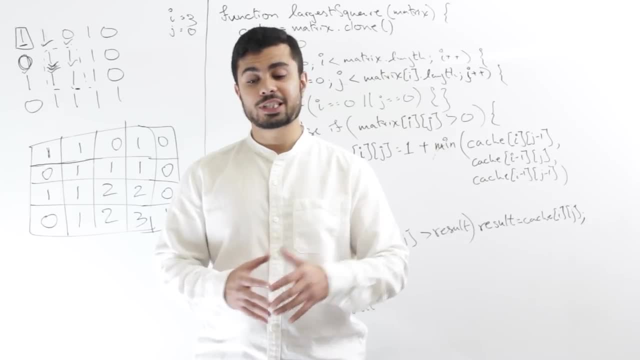 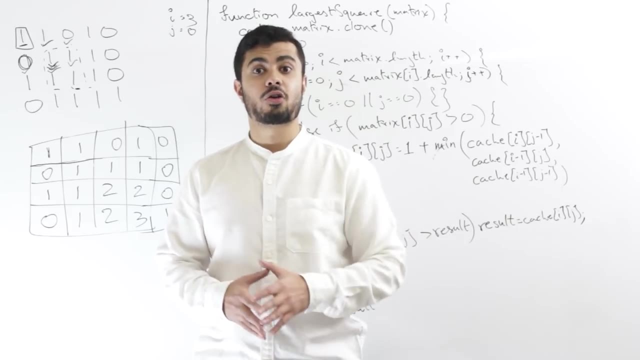 If you want to know or just get updated when it comes out, sign up on the link below and I'll let you know. And next week I'm going to cover the problem where you have to find the maximum area of rectangles inside of a histogram. So I'll see you next week.